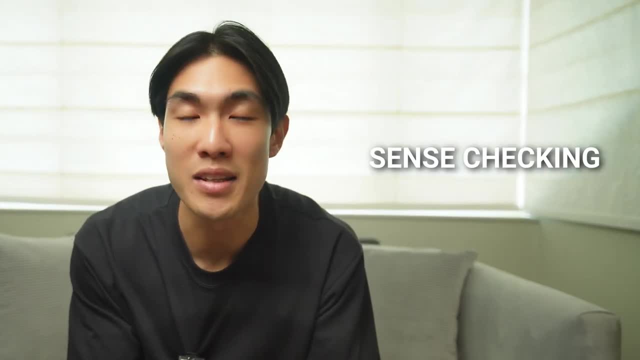 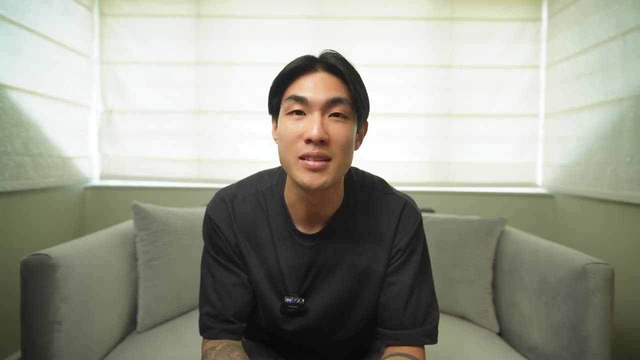 To the case study, Since checking the data is the first thing I do. What file format is my data in? CSV, Excel, JSON, something else? What data is it that I'm working with? In our case, the dataset is a bank customer churn dataset from Kaggle. It's a comma-separated file and each row of data belongs. 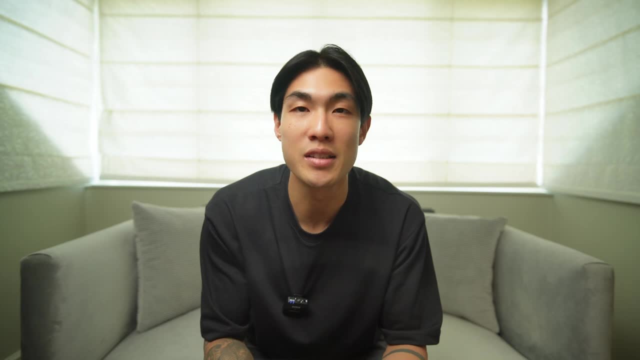 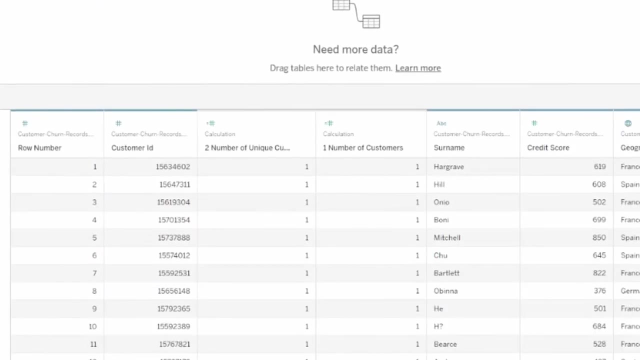 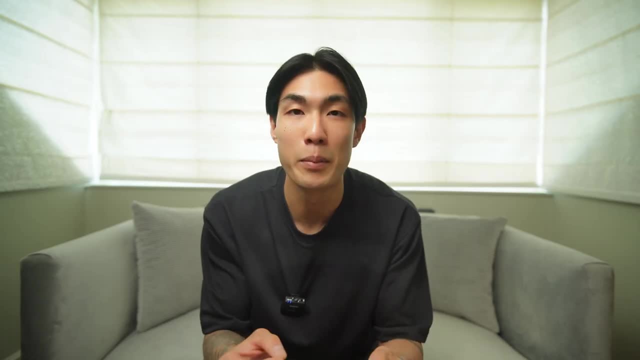 are present in each column. I take my time familiarizing myself with the dataset, as it's happened numerous times before in my career that I jumped the gun too quick, only to realize at the end of my analysis that I used the wrong column or I could have used a different, more suitable 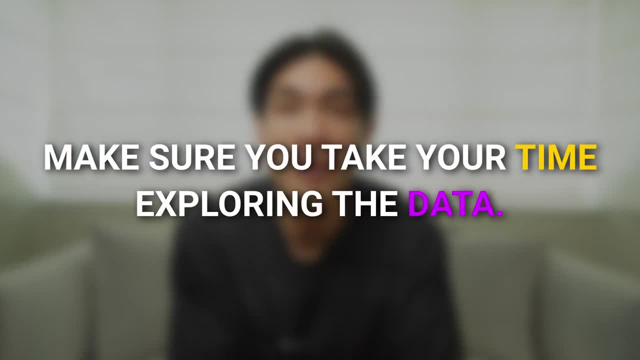 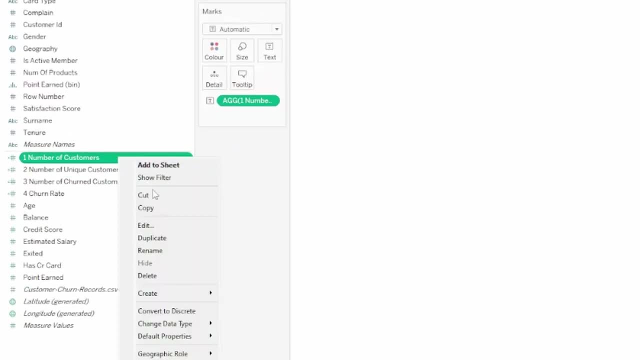 column for the calculations. So make sure you take your time exploring the data so you know exactly what to use and look for the data that you're looking for. If you have any questions, feel free to ask them in the comments below. I did a quick sense check on the number of customers and 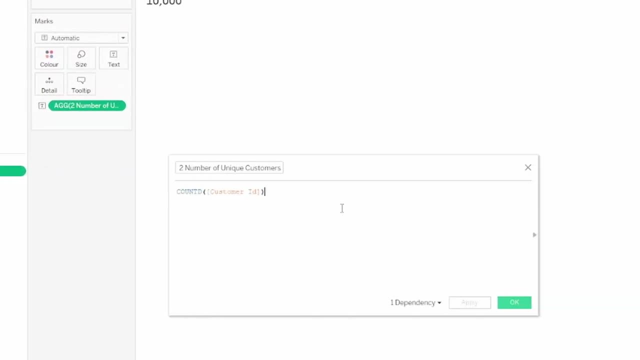 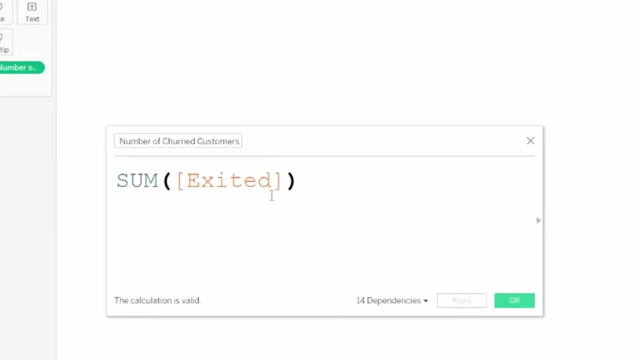 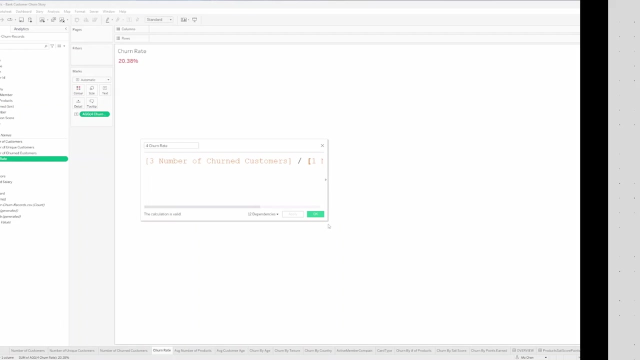 the number of unique customers here, to check that each row indeed represents a unique customer. Then I summed up the number of churned customers, which are just the customers who have already left the bank. Then I calculated our key metric, the churn rate, which is the number of churned. 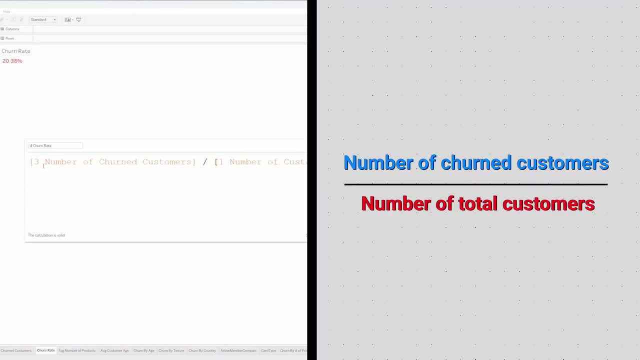 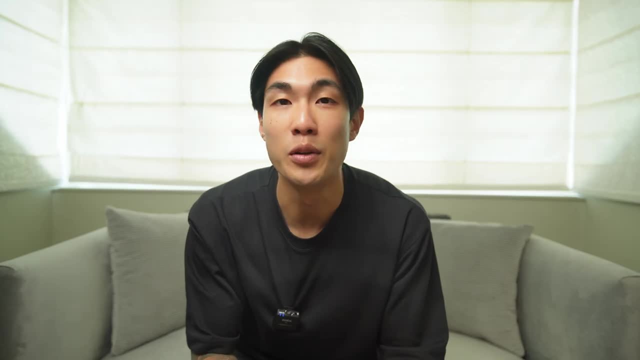 customers divided by the number of total customers, You can see that I numbered all of my calculations. so if you decide to download the workbook, you'll know the order in which you have to do things. I also calculated the average number of products the customers have with the 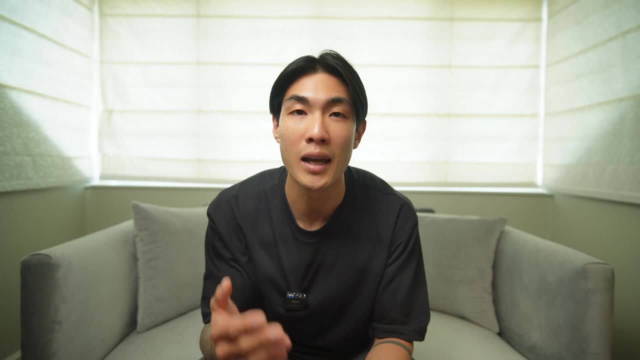 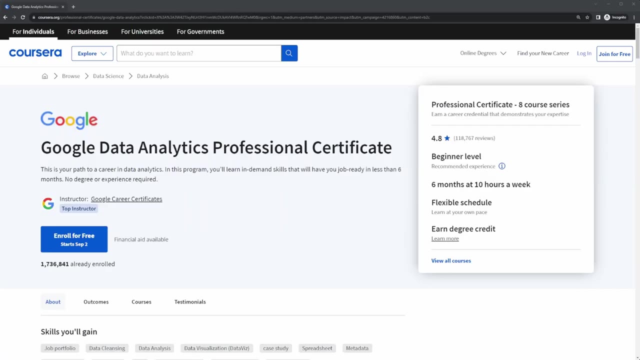 bank and the average customer age as well, to provide more high level context. If you're interested in more case studies like this one, Coursera's Google Data Analytics Professional Certificate would be a great choice for you, as you get to learn in-demand data analyst skills. 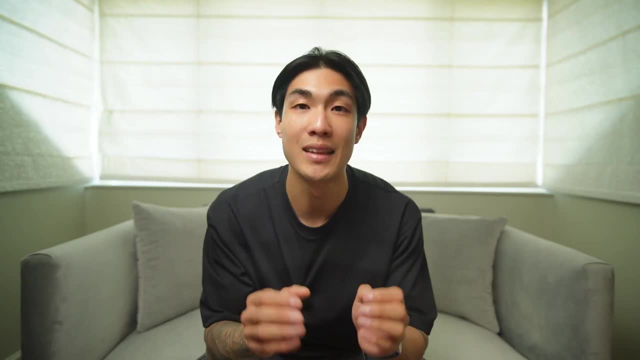 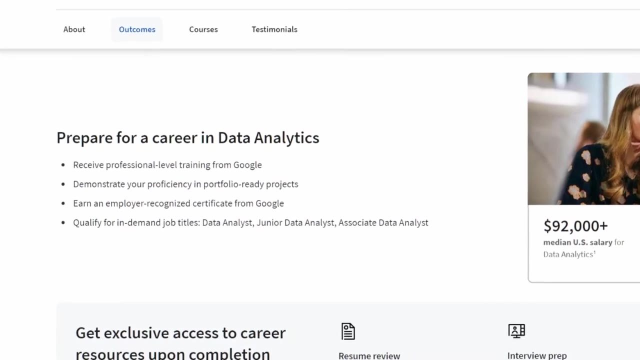 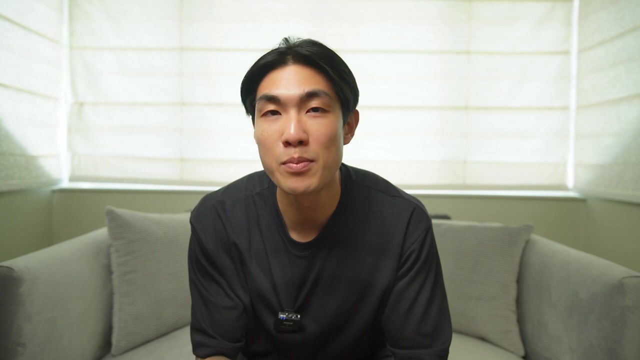 in less than 6 months. if you invest 10 hours per week, You'll learn key analytical skills, from data cleaning to data analysis and visualization, and how to use platforms and tools like spreadsheets, SQL Tableau and R programming. To me, the best part about the certificate is definitely the. 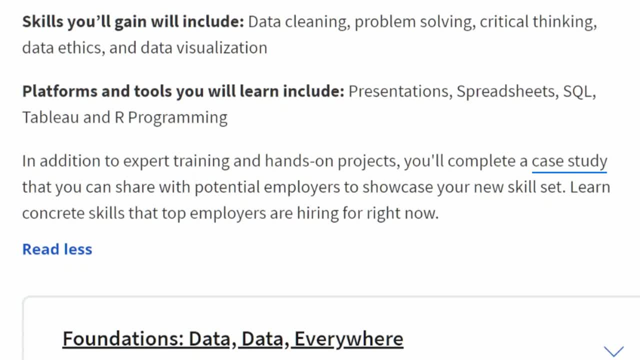 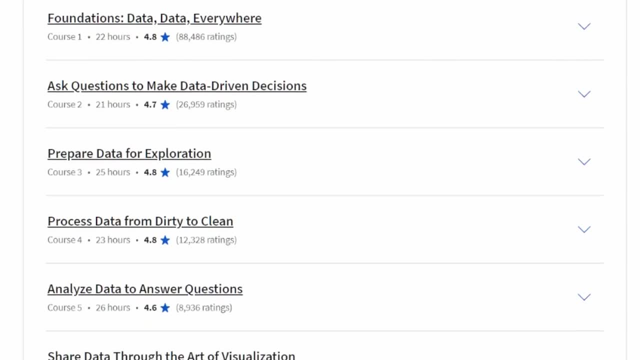 hands-on projects and the case study at the end that you can share with potential employers to showcase your new skills. You do not need previous experience to start this program. it is 100% online and you can take it at your own pace Once you've completed the certification. 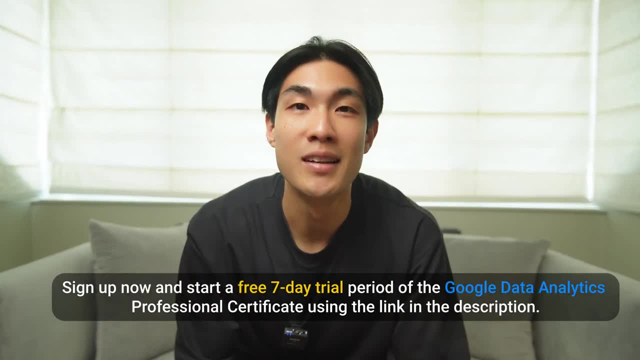 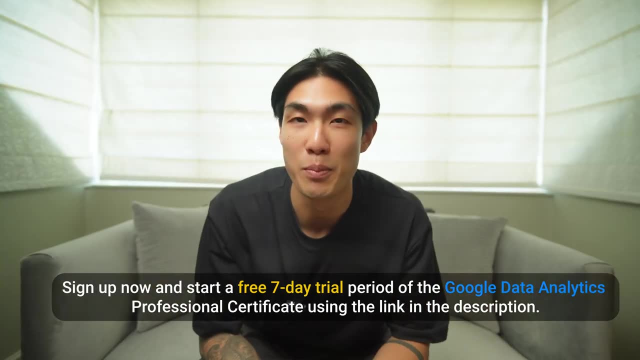 you can add it to your CV and LinkedIn. If you're interested, sign up to start a free 7-day trial of the Google Data Analytics Professional Certificate using the link in the description below. After getting some summary metrics, I decided to dig deeper by looking at churn rates across. 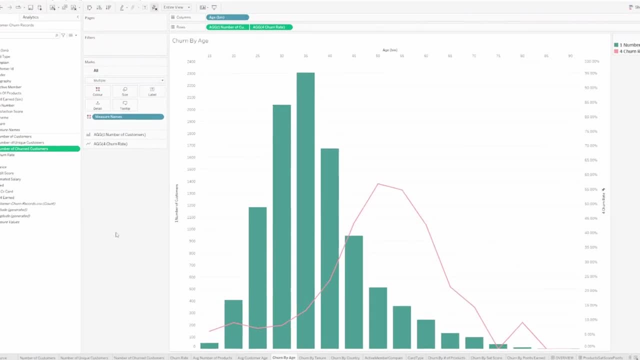 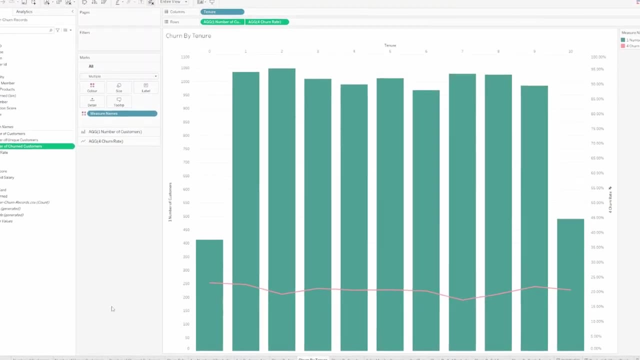 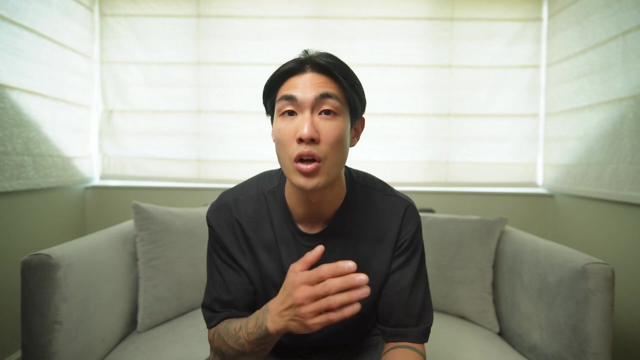 age and tenure. I could instantly see that people between 45 and 60 tend to leave the bank at a much higher rate than other age groups. I could also see that tenure- the years the customers have been using the bank for- doesn't really impact churn rates, as they are relatively constant across all. 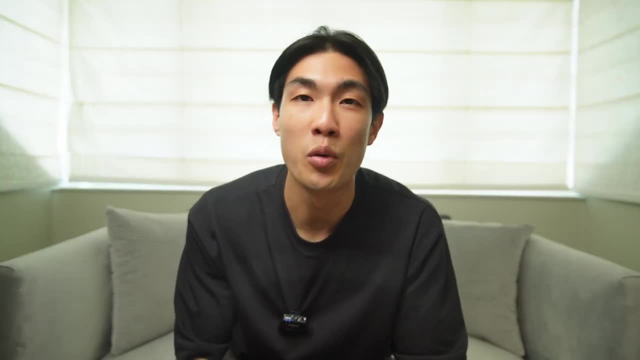 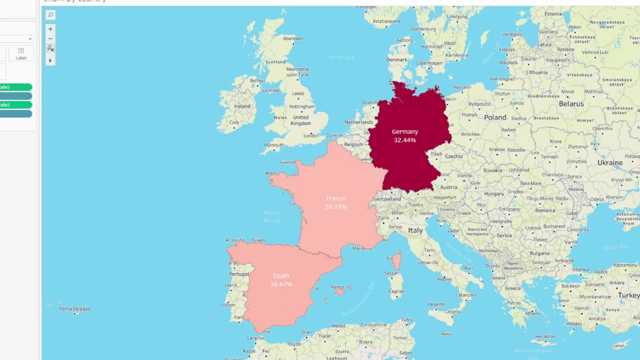 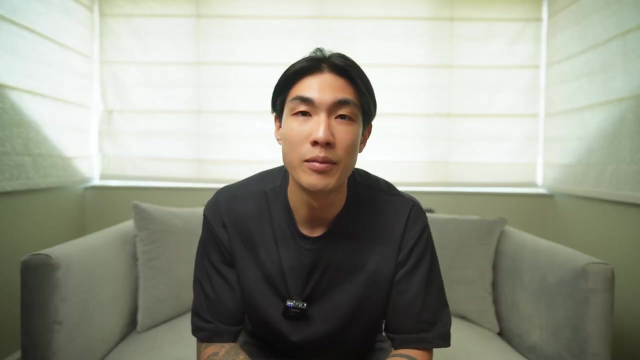 tenures. Then I decided to explore whether there are any geographical differences based on the country column. I used a map to visualize the churn rates by countries and the higher churn rate in Germany stood out immediately, Basically doubled out of France and Spain. I used the is active member and complains columns to prove a hypothesis I had, which is that 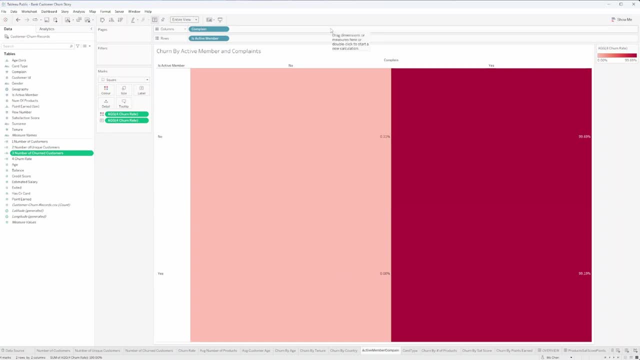 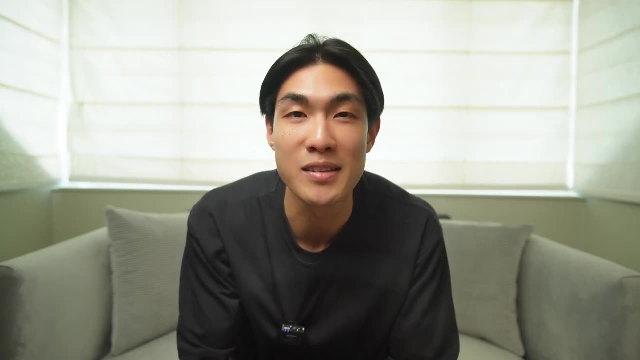 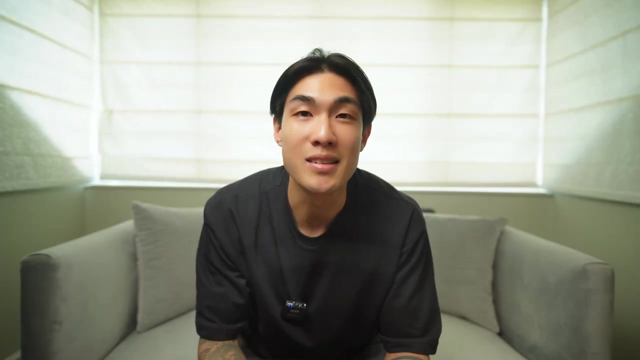 customers who are active and have not complained are much less likely to leave the bank. Pretty common sense stuff, I know. After creating this mini heat map, I proved myself right: Active customers who have not complained at all have not left the bank- Not one of them- Whereas the 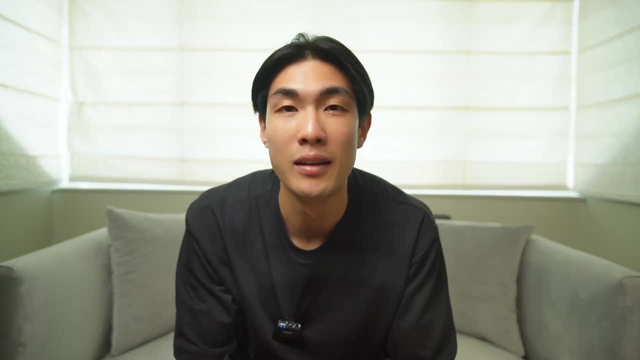 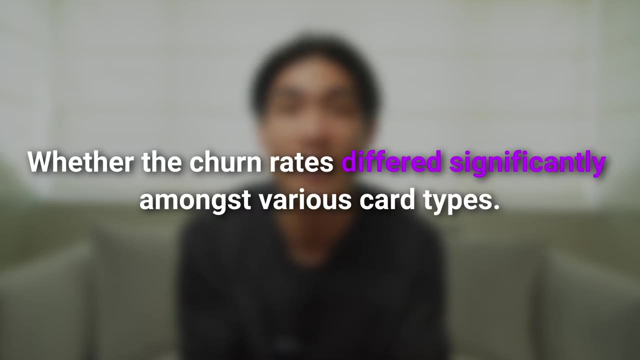 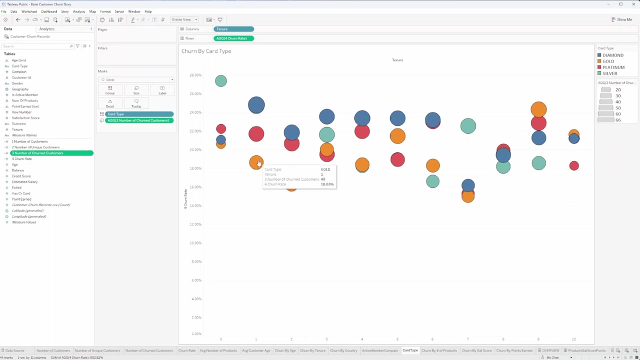 inactive. customers who have complained have pretty much all left the bank. Not great for business, is it? My next thought was to look at whether the churn rates differed significantly amongst various card types. I created a scatterplot with the colors representing the card types, the number of churned. 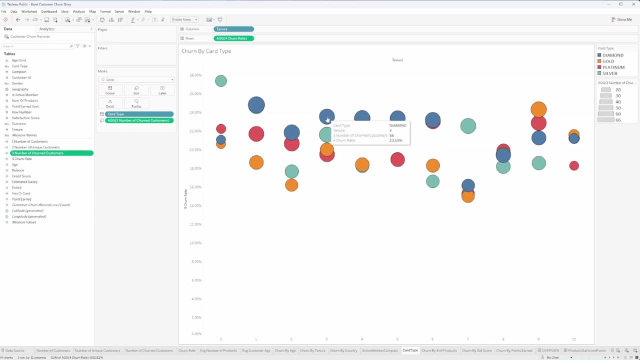 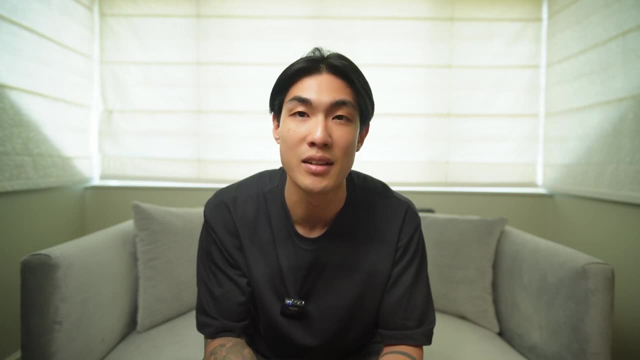 customers the circle size, with the churn rate on the y-axis and the tenure on the x-axis, I came to the conclusion that, for the customers who have been with the bank for at most seven years, churn rates tend to be lowest for gold card types and highest for diamond card types.